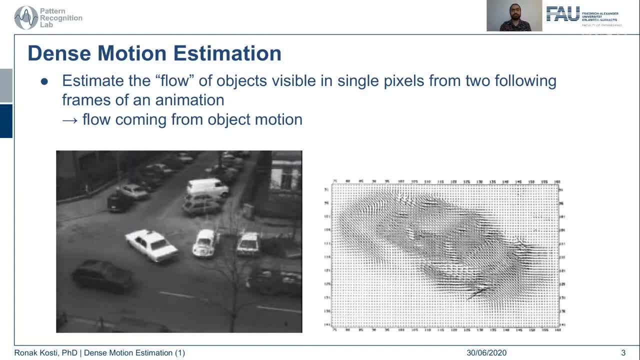 Usually the flow or the motion that comes from either the object moves or the camera moves. So if you are changing the position or location of your camera, then there is an apparent motion, or if the object itself moves, when the camera is steady- In this case, for example, on the left hand side. 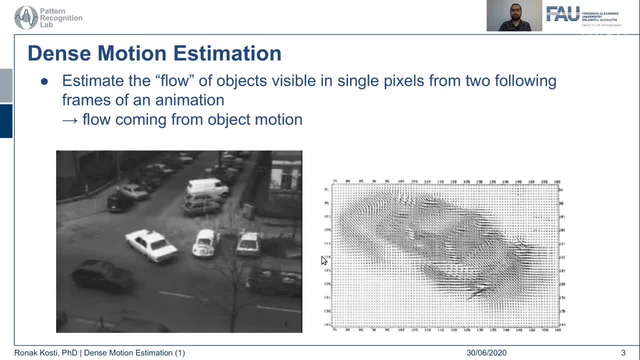 you see a car here and this is a flow field or the flow of generated by this car in a small video. How do we determine this flow? is through some vectors which did which show you the strength and the direction of this flow around this object, and this kind of flow field generate. 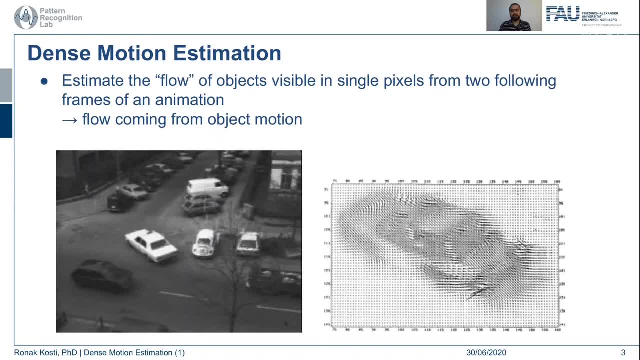 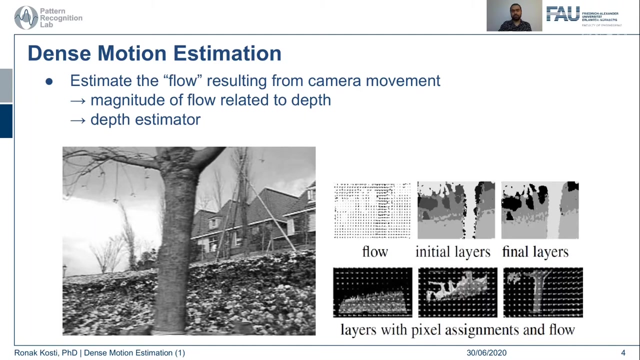 generated flow field is called motion estimation or a flow of this object. Basically, we are trying to quantify the object motion in computationally and that's what we call as flow. Okay, and another reason where the flow can also come from is camera movement. So if your image 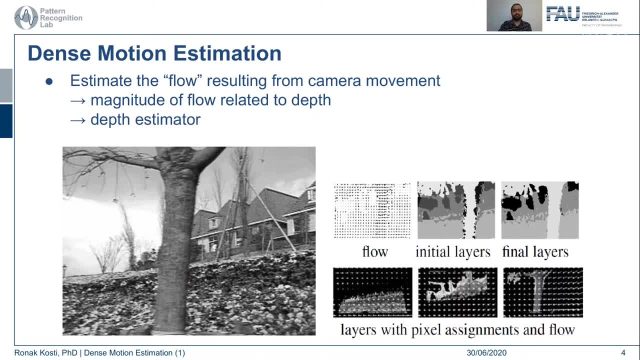 is stationary, and if you generated another image just by moving your camera, then the flow can result from that as well. By estimating the this flow, we can estimate the magnitude of or the relative depth of the objects inside the image, and therefore flow estimation or motion estimation is useful for depth estimation as well, As in this case. we can see the flow field here is: 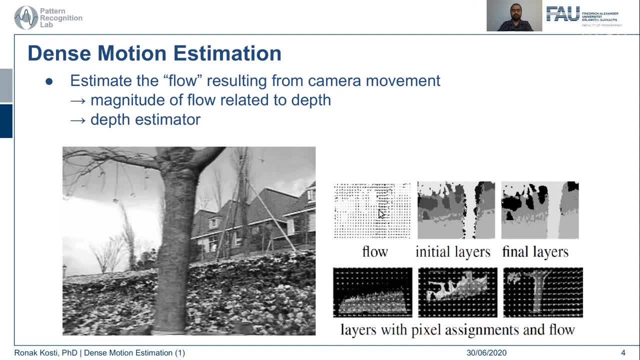 generated and you can see that the higher or the more stronger field are visible in the trunk of this tree, whereas lower or very less magnitude fields are seen in around the sky, areas or objects which are farther away from the camera. and this this is due to the perspective view of the camera, because when you translate or 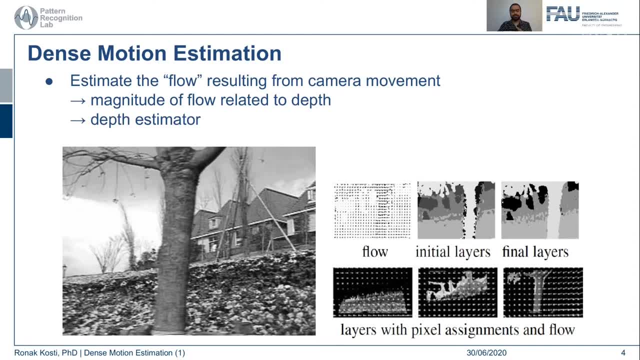 transform 3d object into 2d image plane. the objects which are closer to the image plane will show a higher magnitude of flow or motion estimation or motion estimation as well, And objects which are farther away will show lower values of motion fields typically. 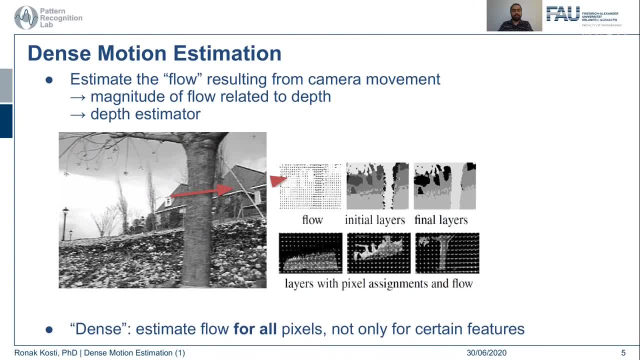 Basically, as you see here, the dense estimate of all the pixel values is considered as dense, and it is not only for one particular feature, like the trunk of the tree or the house, but it is actually for every pixel in the image. There are different applications for generic motion estimation as well as dense motion estimation. 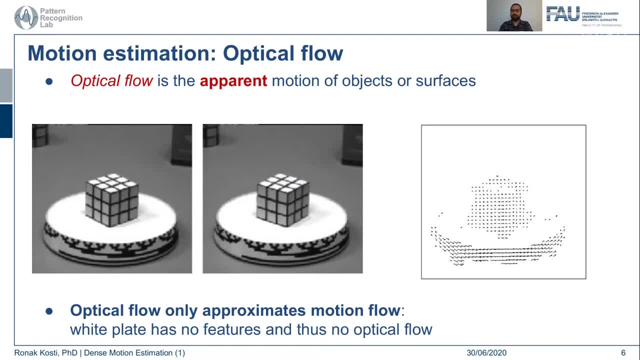 We will see some examples now of what it means to have this kind of a flow or trying to compute this flow. So motion estimation can be also interchangeably be also called optical flow. These two things are used in conjunction with one another more often than not. There is a slight difference between them. 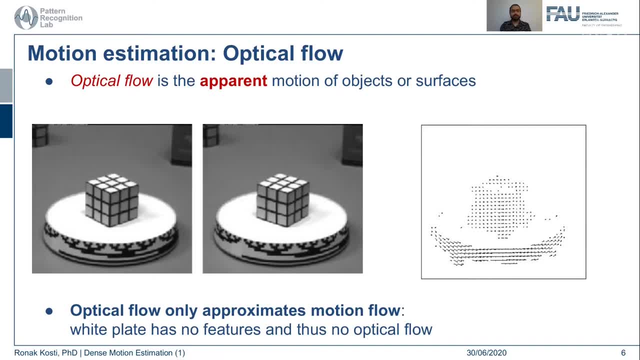 We will look at them later in the slides. But what is optical flow? Optical flow is essentially the apparent movement or motion of objects or surfaces across frames, and optical flow will generate the vector fields, which is just how much, which is an, which is a value. 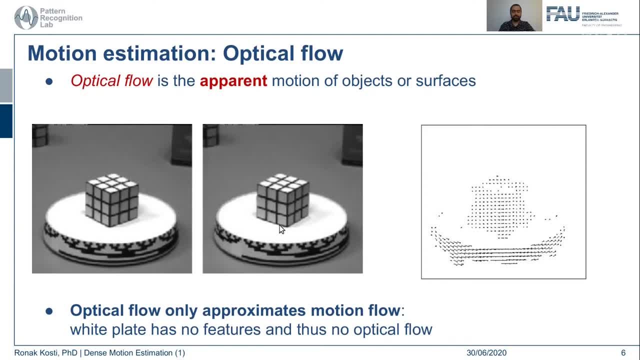 Of how much the pixel moved from one image to the other. another image. In this case you can see a Rubik's cube lying on a white surface and this is like a rotating body here, and you can see clearly that the whole the Rubik's cube, along with the surface, has moved or made a counterclockwise rotation. 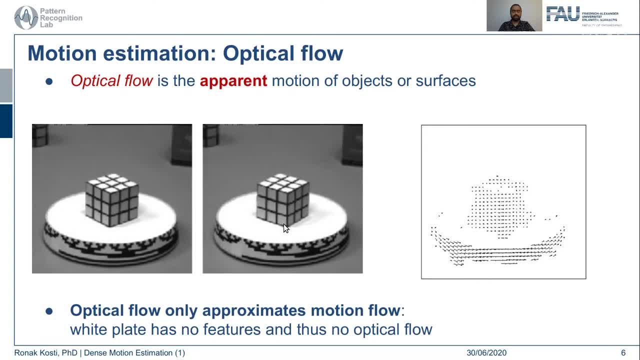 and this is another instance of that rotation. You can see from these features here at the bottom of this plate that this plate has moved along with the Rubik's cube. here, However, we optical flow is able to only detect the apparent motion of the 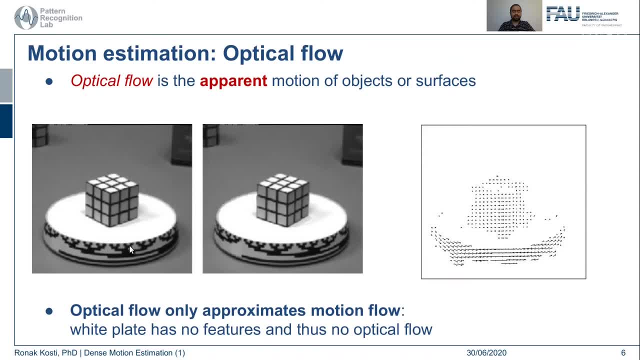 Rubik's cube and the features which are visible in the bottom of the plate. but there are no visible features. It's basically a white surface on this plate and therefore there are no motion fields or optical flow estimated for that. We know that the plate has moved but because there is an absence of features there, optical 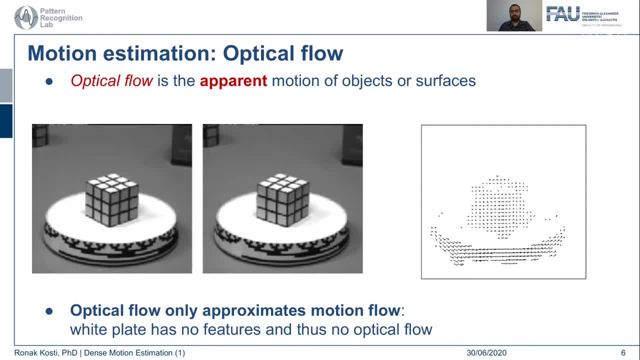 flow, was not able to estimate the flow for these surfaces, Whereas in case of Rubik's cube, it is clear that the Rubik's cube- here, if you zoom in and see, you will see a lot of the errors pointing on the right hand side, showing that. 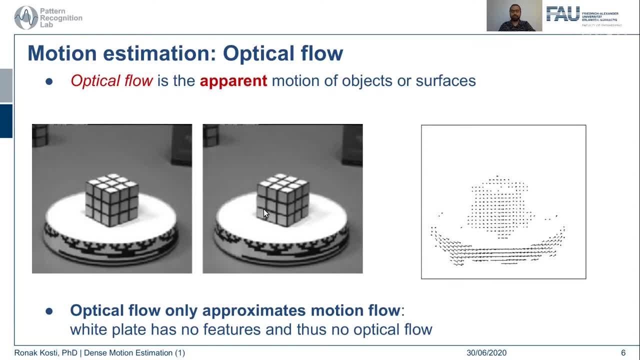 the object has moved from one image to the other. on the right hand side. Similarly, at the bottom of the plate, you can see that there are optical flow with higher magnitudes oriented towards the right hand side direction and anti-clockwise direction, here going towards top left. 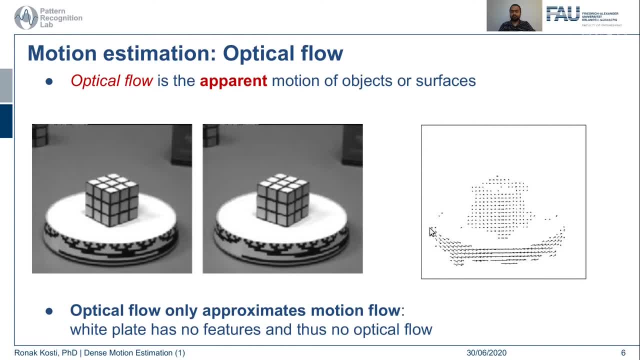 And this on the left hand side of the plate. you can see that the flow is coming from top left. Sorry, here I meant top right. These arrows are pointing towards top right, So, and here you can see that these arrows are coming from the top left. 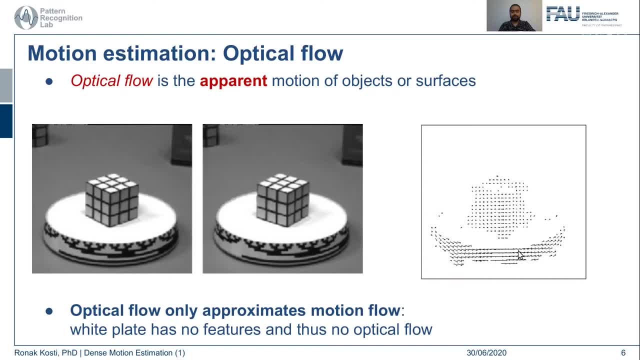 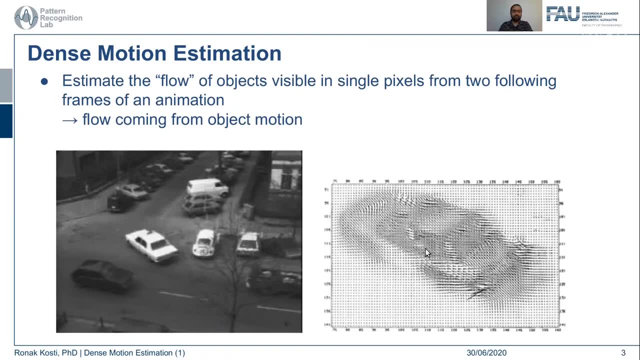 So it's kind of showing you how the plate has moved in an anti-clockwise direction. Similarly in the case of the car. here we also see that in some parts of the car where there are white surfaces it's not easy to locate or estimate the optical flow. 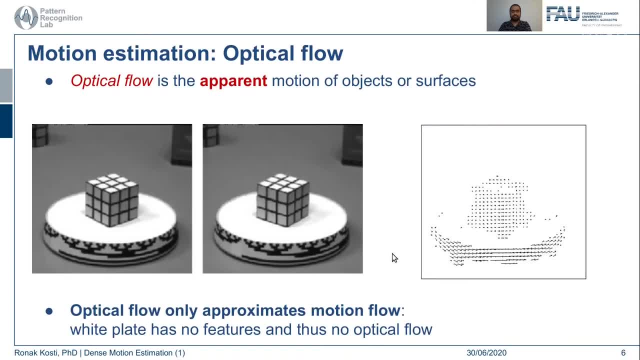 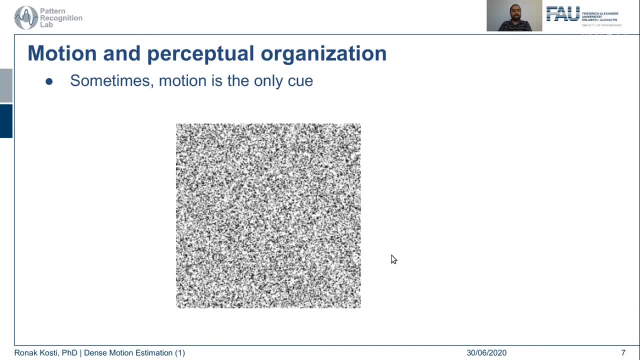 So optical flow really relies on features present in one image too. Okay, I'm going to try to show you how optical flow works over the other image And motion sometimes is the only cue and it's not so easy to see for the machines, but for 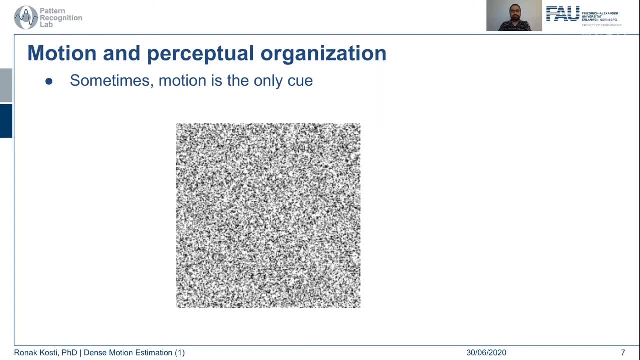 us. it's quite simple to understand or visualize this motion. For example, in this case, you see an image of noisy pixels here. Now, if you saw that there is an apparent motion from one image to the other, you can the other. you can see that there is a square in middle which is moving right. 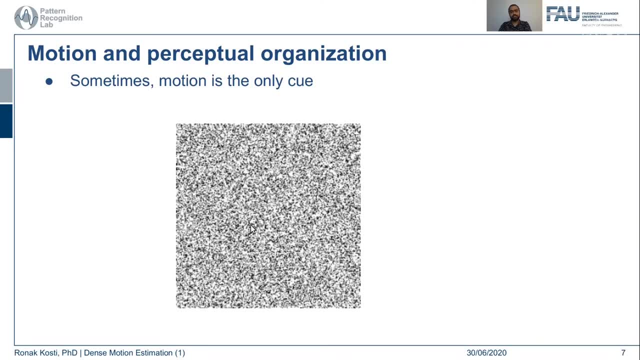 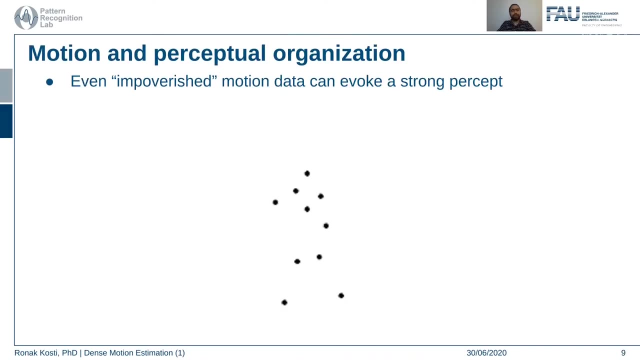 it's quite easy for us to see, but for a machine it's not easy to see, and this kind of perceptual motion is also important and has to be considered while doing motion estimation. I want to continue by talking about some perceptual motions. so, for example, even if we have data like this, where there are some 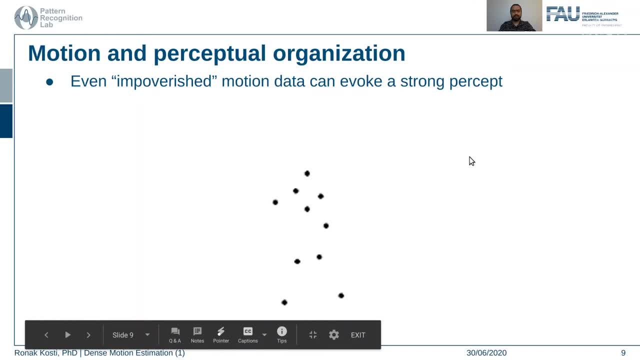 random points visible on the screen, however it's, it could be random points, but when you look at, when you show some motion along this point, you can see an apparent moment here that it's a motion of a person walking. and this kind of perceptual motion is possible even with 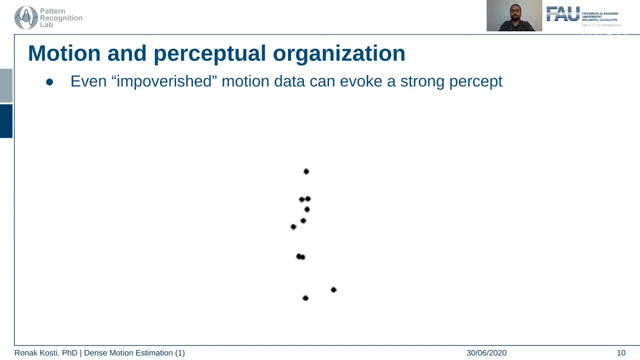 perceptual motion, we can see that it's a motion of a person walking, and this kind of perceptual motion is possible even with a minimum amount of data, and it can give us strong estimates for motion as well, and this also need to be considered while doing motion estimation. and yeah, 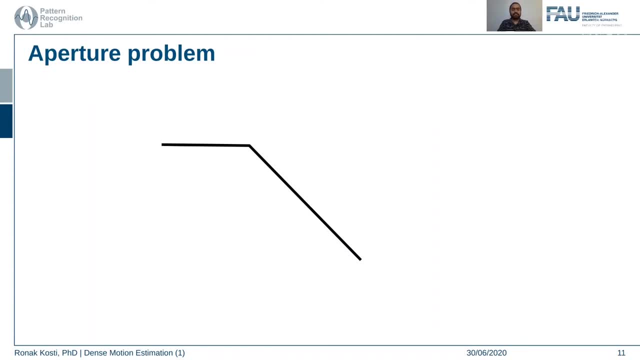 so what are the problems generally faced for motion estimation? or one of them is aperture problem. so what does it mean? so aperture is this opening of the camera with which you are capturing the image, and if you are only recording a certain part of the image and not able, 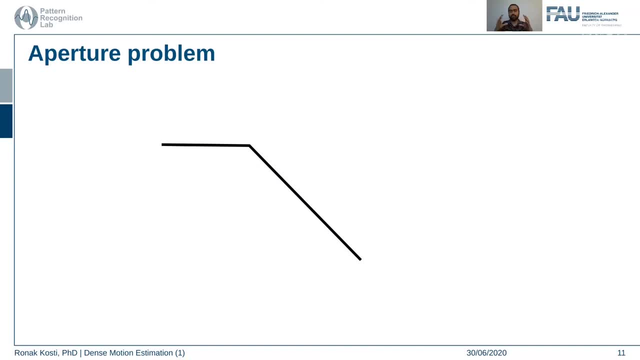 to see the whole image in context, or the whole or a more broader view of the image, then you can have a mis-estimation or a wrong estimation for the motions, completed motion, for example. here this line has this shape: has moved on the right hand side. 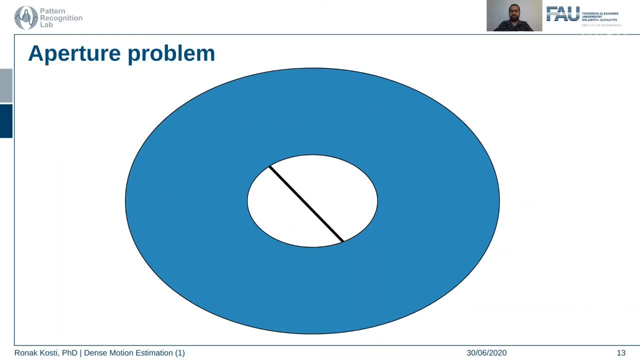 whereas if we look through the aperture, for example, in this case we see that the line has moved from the bottom left to the top right, which is not the case. right, the case is that the shape has moved on the towards the right. so this is one problem faced by motion estimation. 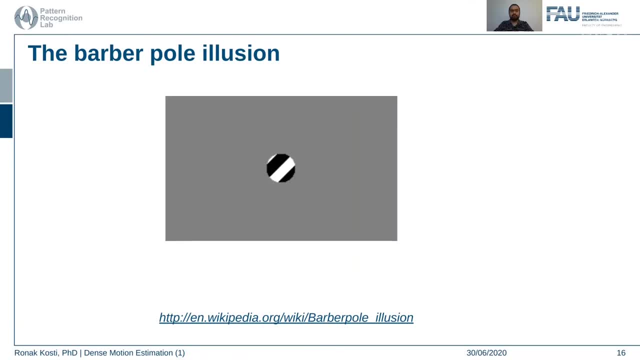 another one is called the barber pole illusion, which is similar to the previous one. If the aperture or the field of view is very low here, it can give you a wrong motion information as well. What's happening here is we see that there are some lines which are moving from the top left towards the bottom right. 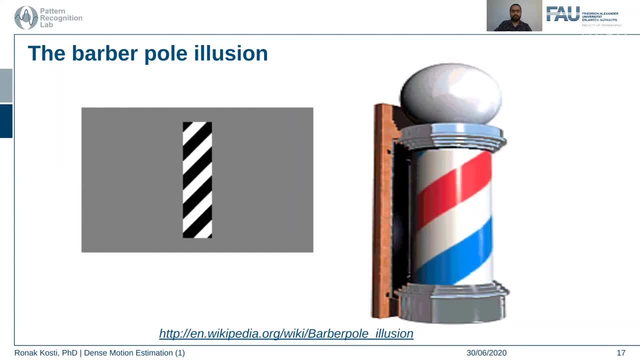 However, they are simply rotation over a cylinder And if you are looking at it from an aperture perspective, from through a particular small size, fixed size aperture, it can give you a perception of movement in the wrong direction. So the barber pole illusion is another problem that can be faced for motion estimation. 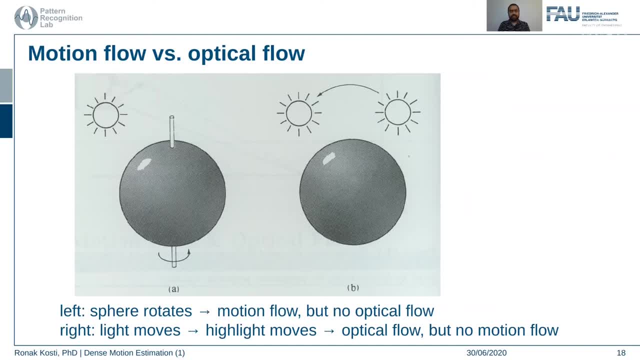 Okay. so before this we saw how we were Using motion flow and optical flow interchangeably. Here we will focus a bit more on the same aspect. So motion is associated. motion flow is associated with the objects themselves if they are moving. 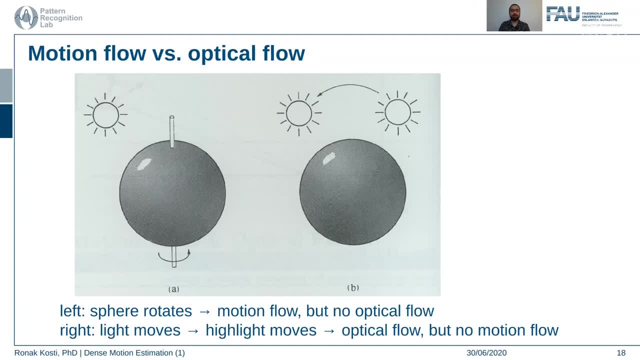 And optical flow is the apparent or the perceptual understanding of the motion. Basically, if we see some features moving, then Can we compute that or not. that is in from a computational sense. that is optical flow. however, not necessarily the object has to move in that case. an example here is: on the left hand side you can see a sphere and you can see the reflection of the sun on the sphere, and this sphere is quite smooth, with uniform surface reflectance, and it's moving in the counterclockwise direction. 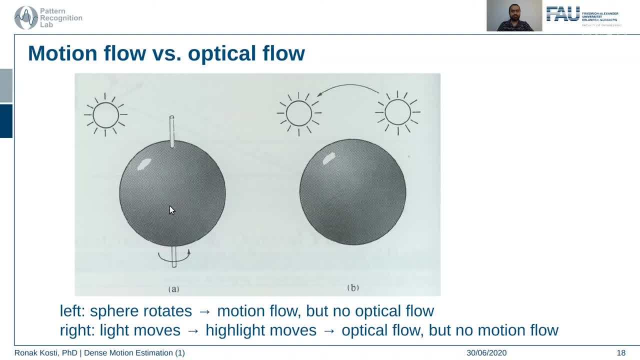 So here there is a motion flow of the object, whereas there is no optical flow, because this reflection will not change And even though the sphere rotates, there is no optical flow. on the other hand, on the right hand side, there is a movement of the sun, whereas the sphere is fixed. 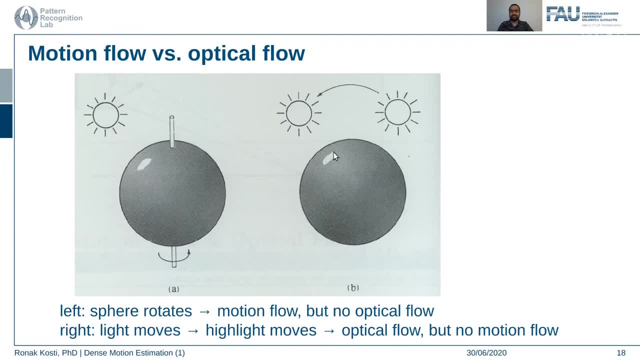 So what we see here is we will see here is that this reflection will move from this point, So over somewhere here, and this will create and apparent optical flow, but the sphere is fixed, So there is no motion flow. This is the basic difference between optical flow and motion flow. 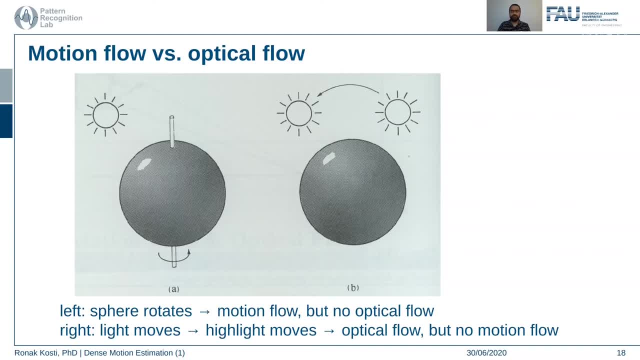 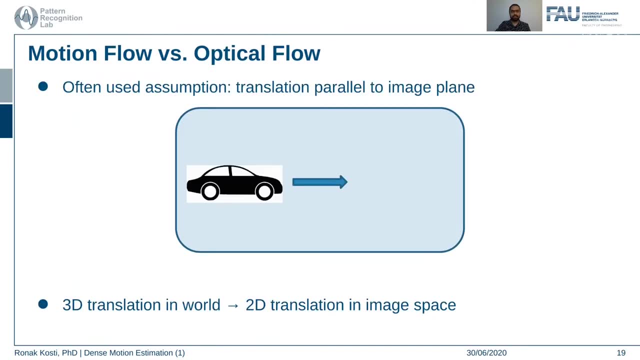 Depending on the application. you have to consider what we can use or what we are aiming to estimate. Another example of the differences between the optical flow and the motion flow. flow is is an often used assumption is that translation is a parallel to the image. plane will give us a wrong perception sometimes. so let's say if 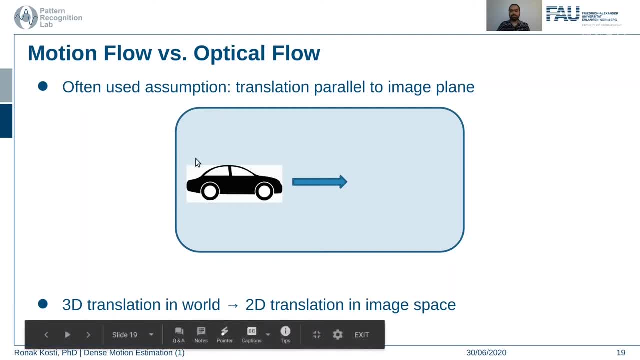 your car here. this is your image plane, and your car moves from this point towards the right hand side. here, all the pixels in the car are moving in one direction, together in with the same magnitude, so every point has moved with a fixed magnitude. on the right, however, this is this assumption is not true, or? 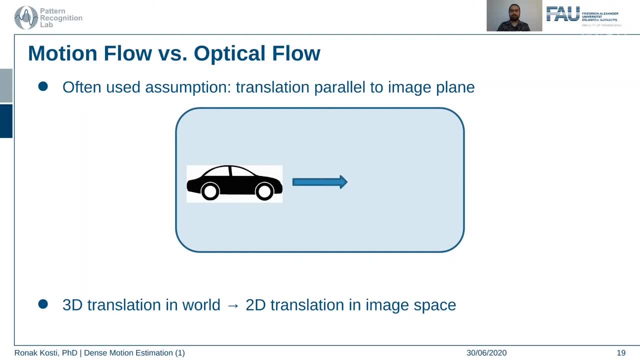 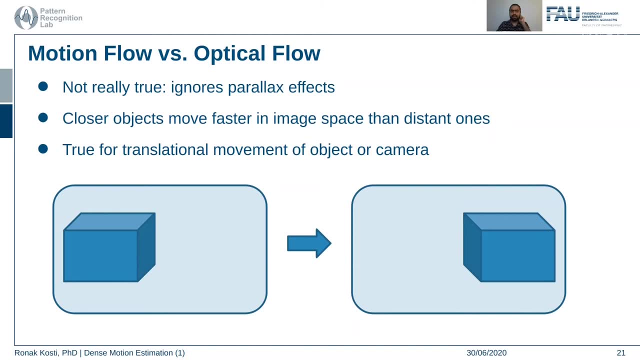 in every case. sometimes we have, we make this assumption, but this incorrect, because we will see why- because this kind of motion or this kind of kind of assumption ignores parallax effects. what do we mean by that here? so let's say there is a cube here which moves on the right hand side like 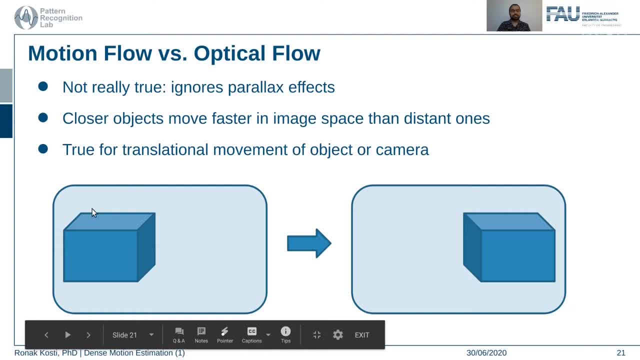 this now. but due to parallax, the depth or the objects or the parts of this square or the cube which are away from the camera give a lesser, or travel lesser distance in 2d image plane than the surface points which are in the front of this cube. so you can see. 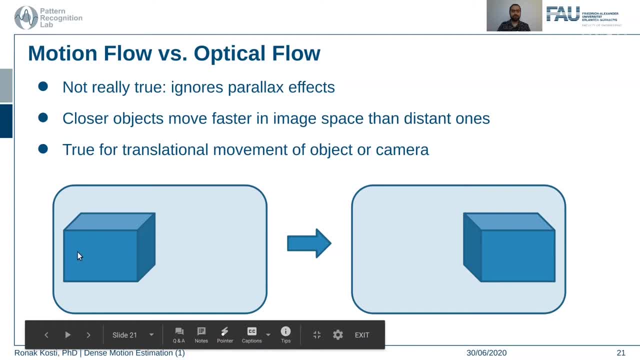 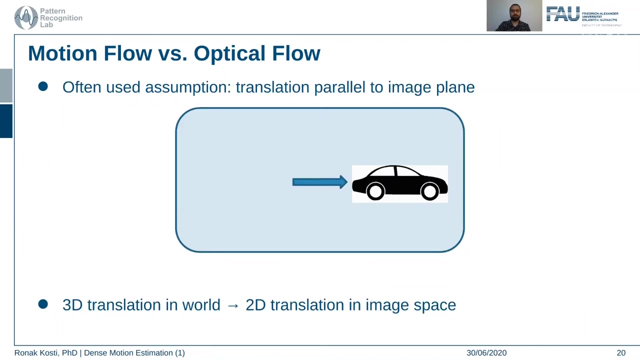 that the objects or the points which are closer to the camera have moved longer or more further than the points which are in the behind or at the far end of the cube. so there is no, so if there is a, so we cannot make this parallel, we cannot. 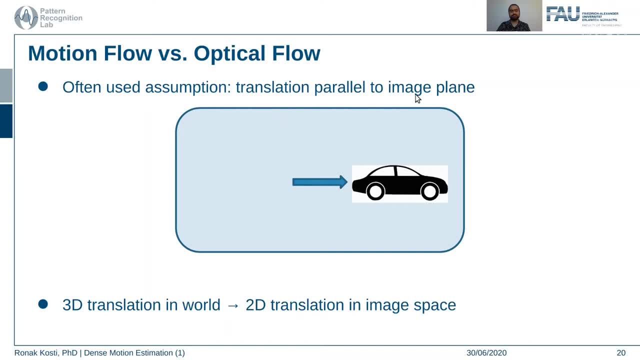 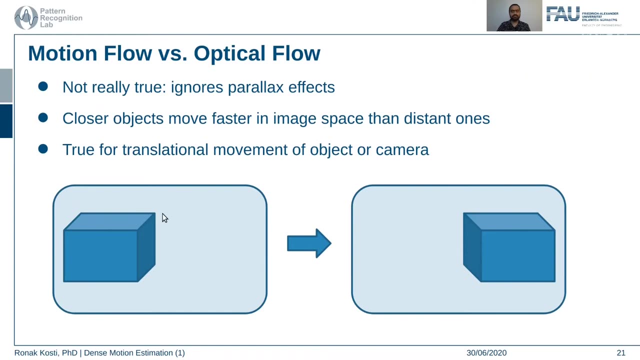 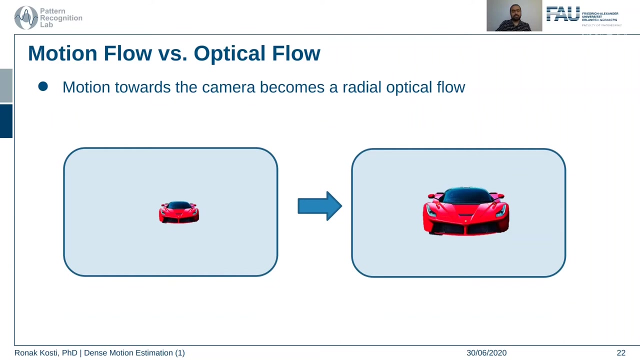 make this assumption of that translation, which is parallel to the image plane, and we'll always move all the pixels in the image with the fixed magnitude, which is not true. closer objects move faster and distance one distant ones move slower. another issue or another aspect of motion is when the motion is towards. 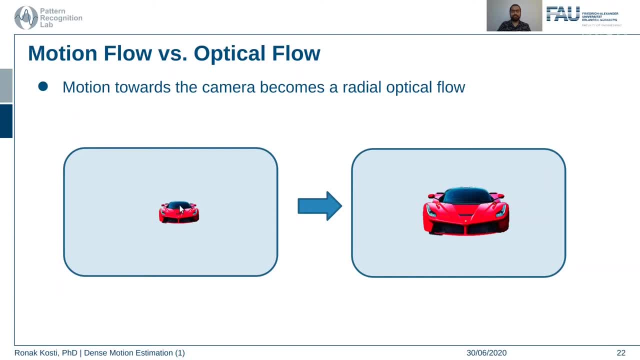 yourself or away from yourself, for example. in this case, this car is moving towards you or towards us and because of this we generate a radical or a radial optical flow which is going away from the object. this kind of optical flow does not give us much information, but we, because we know that this kind of motion can- 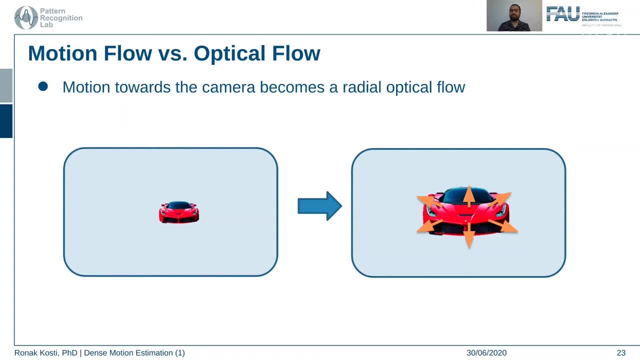 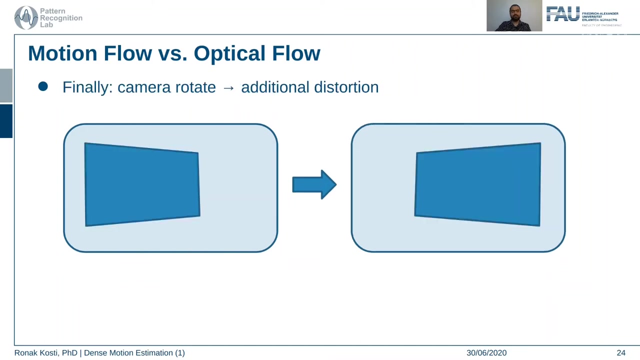 generate this kind of optical flow. we can safely assume that this object is is probably approaching. in the reverse case, if the object was going away, the optical flow vectors will be directed inside and this kind of motion becomes a radial optical flow. basically shows us a radial optical flow. another issue is: 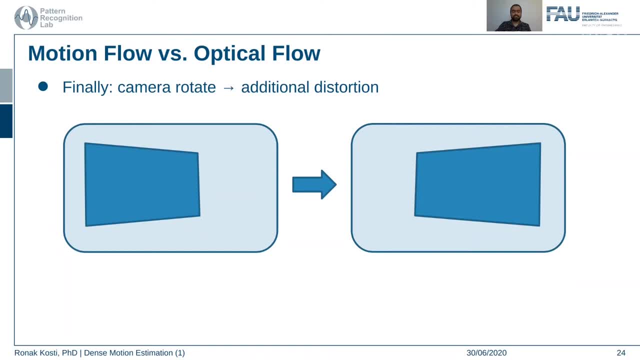 that if you fix the, so if there is a movement of the camera around in a rotational form, for example, here you are taking an image of this rectangle from the left hand side towards the right and take the same image of the square from the right hand side- then 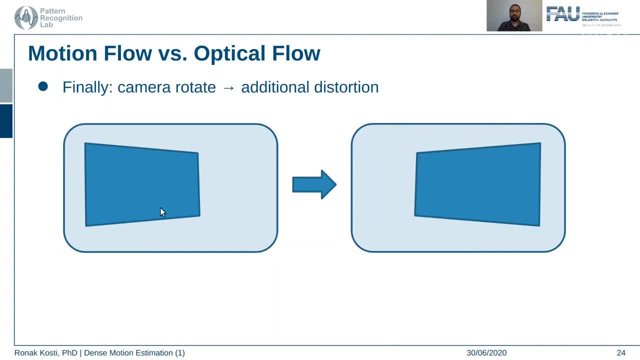 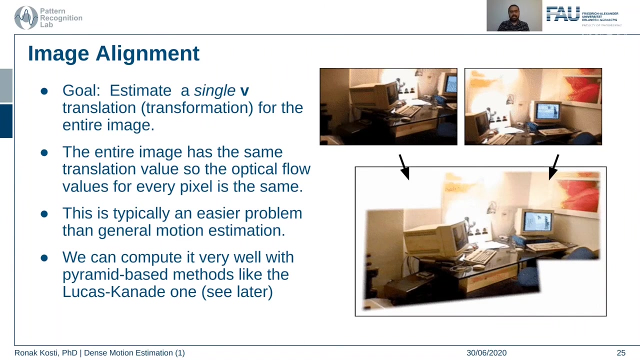 there is no direct translation, where each and every pixel has moved with a fixed motion or fixed magnitude. So there are different aspects to motion flow, as well as optical flow, when considering to compute the motion flow. One of the applications of motion estimation is image alignment. 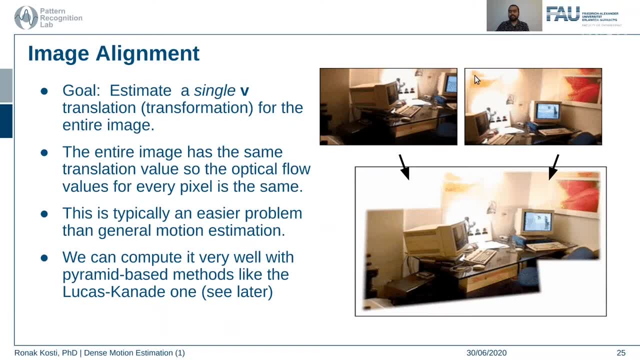 Here our aim is to align two different images taken at taken, two different images captured of the same scene from a different perspective. So we want to basically generate a single V translation for the entire image that translates this image towards the right hand image. So here, assumption. 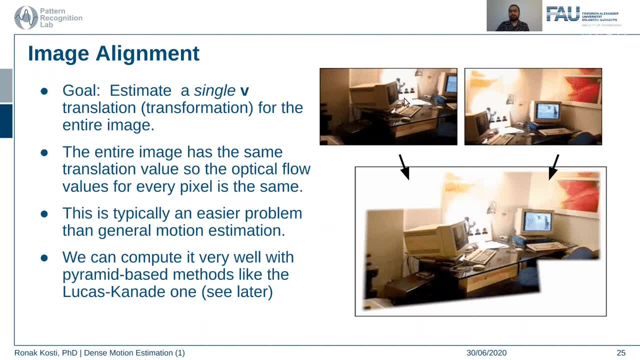 Again, here we make the assumption is that the entire image has the same translation value, so the optical flow values will be the same for each and every pixel. And this is typically an easier problem to solve than general motion estimation, because here we are assuming some fixed values of the optical flow. 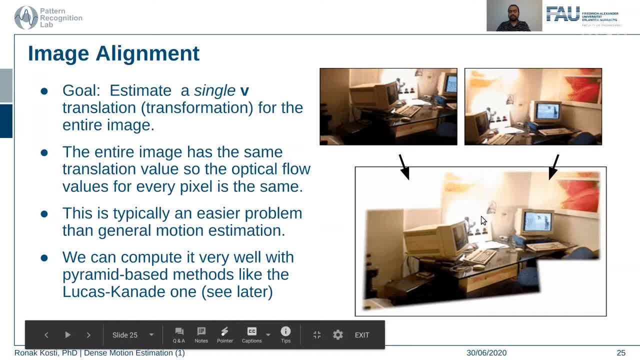 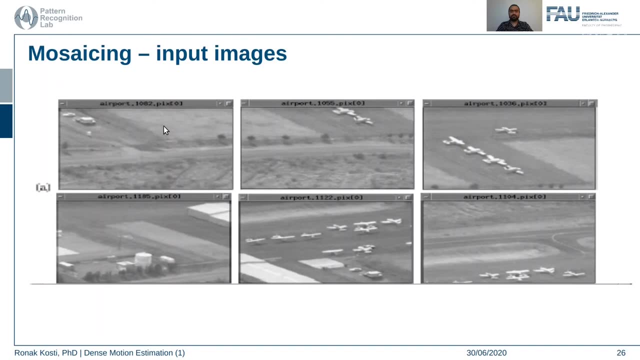 And using Lucas-Canady methods, we can easily compute this kind of image alignment, where you can join different images. Another application is mosaicing or input images, where you have different images taken from. So these are a set of different images taken from a drone of an airport apparently across. 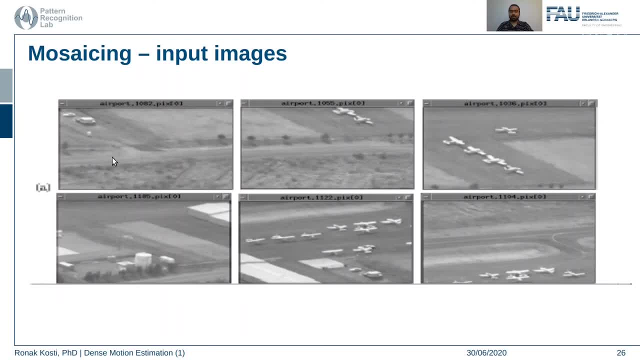 six different frames and because these all objects are quite far away from the camera, so their depths or their distances from the camera are assumed to be constant, although it is not, but given the high altitude of the image capturing device- the drone in this case, for example, is quite large than the inter pixel. 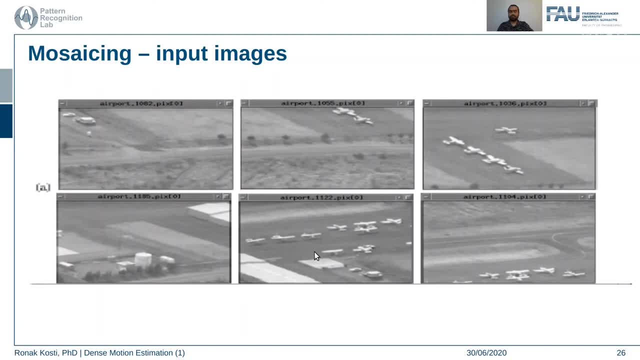 distances between the objects lying. here it is safe to do the or assume that kind of assumption, And so, using the, this information, we can compute or join these images. For example, here you can see this: on the right hand side this image feature overlaps with the right hand. on the left hand side of this image feature. similarly you can see for every: 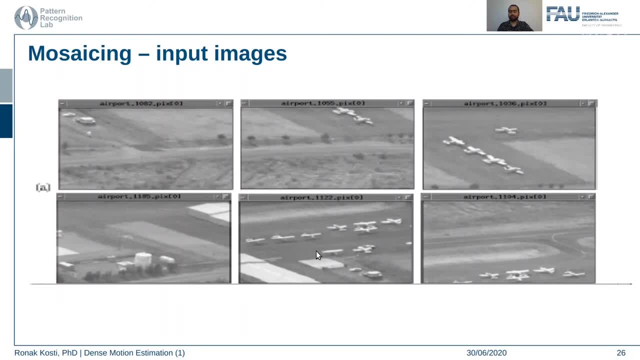 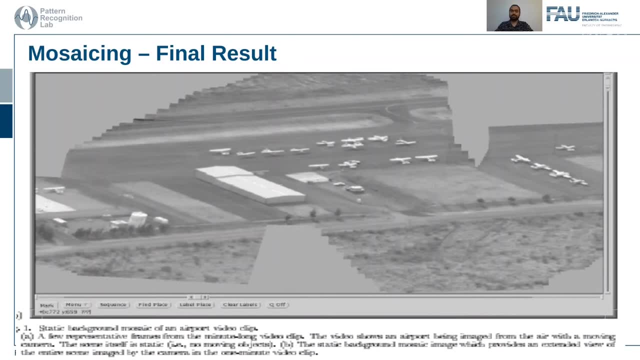 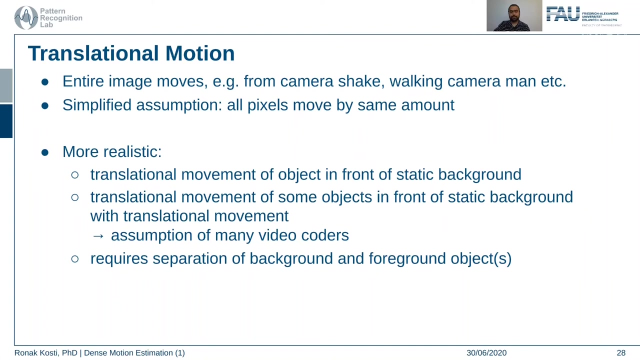 image. you will find some overlap of one image over the other, and then you can just do a stitching of this image where you can generate a final mosaicing, which is a simple and straightforward given the assumptions that we have made. Okay, so what we have talked about is a basic translational motion where we have assumed 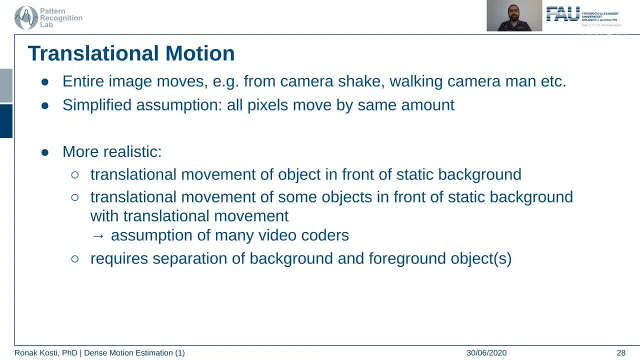 the optical flow values to be constant across entire images and one of the application is as image stabilization, where you are taking an image of an article, an image of a scene where you have a small shake or a movement of your camera, where the assumption is made that all the pixels are moving with a fixed value and therefore the new cameras, what? 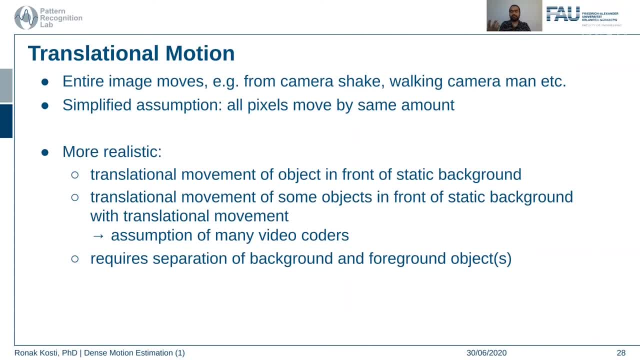 we have now even in your mobile phones have image stabilization software built in, so when you are, whenever you are taking a camera, even with jerks or sudden random movements of your camera device, the image does not get blurred. and this is one direct application of this translational motion. 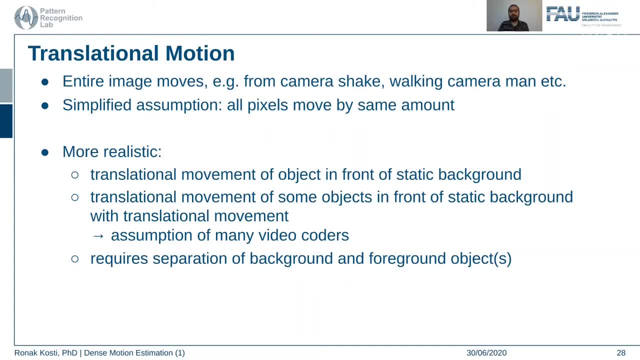 This can happen with walking cameraman for our camera shake, so on and so forth. as I said, simple assumption that we have made is: all pixels move by the same amount. More realistically, if you are doing object tracking or your focus is on a particular aspect of the image, certain feature or certain region, then you have to subtract the background. 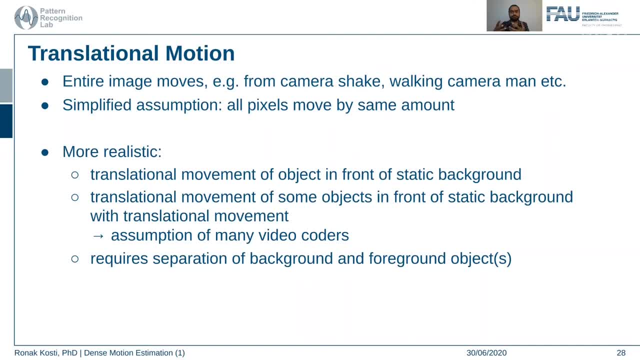 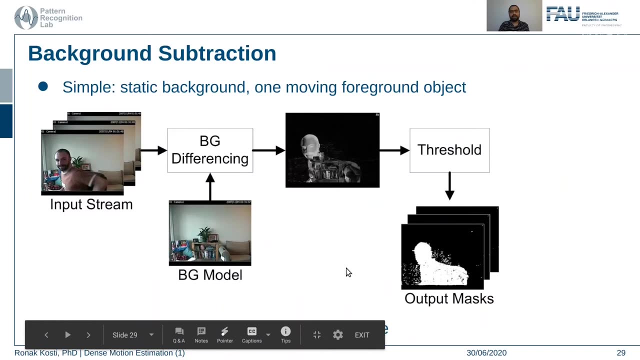 from the foreground Or you have to focus your attention towards the object that you are interested in. for this motion- and this is the assumption of a lot of many video coders- however, it requires a separation of background and foreground objects. One direct application or one direct way of doing this background subtraction is first: 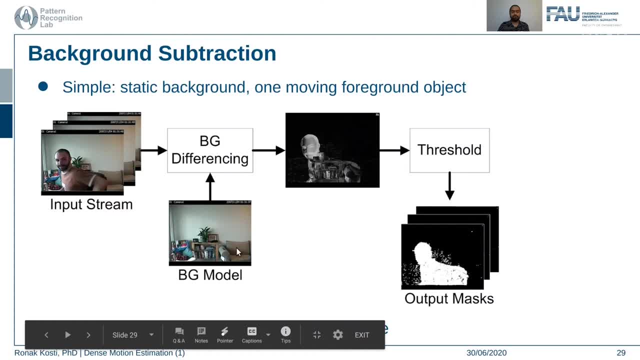 you take an image of the background, so you get a background model and you fix that background And then you start your or insert your object in that. and when you take a difference of this input and the background, you will generate a motion field which is associated with your. 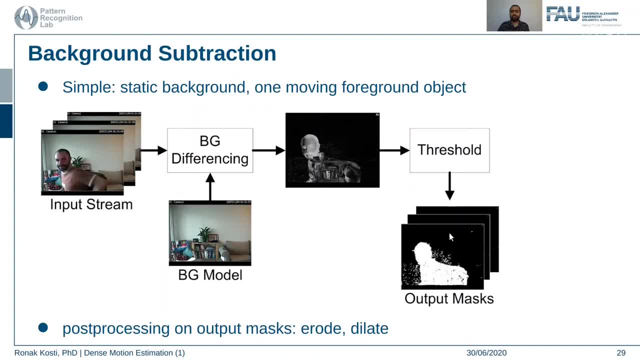 foreground objects and, using proper thresholding, you can generate a mask or a field values which show how much the foreground object is moving with respect to your background And then you start your or insert your object in that and when you take a difference of the background, you will generate a mask or a field values which show how much the foreground 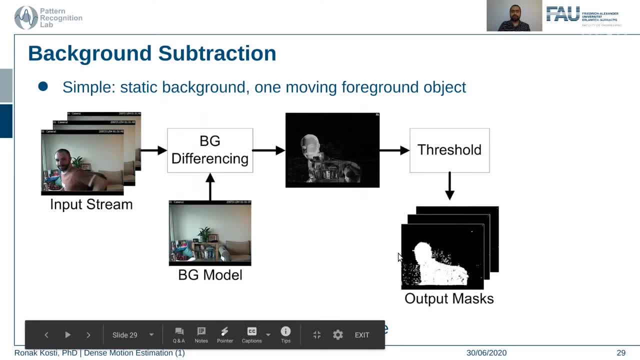 object is moving with respect to your background. The problem with this is that sometimes there is a lot of spurious noise present in the estimation or even during calculating these differences. As you can see, there are some random dots- white dots- visible, and we don't want them. 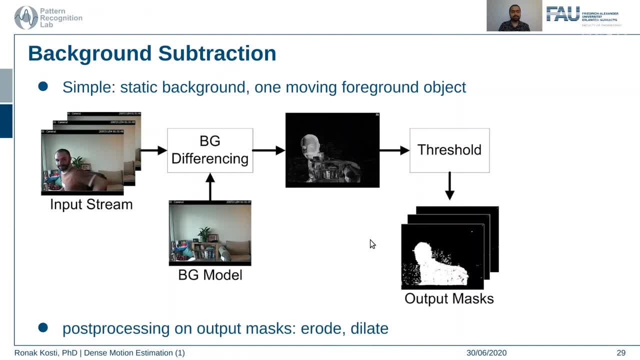 so you do some sort of post processing on those output masks where you use simple image processing techniques like erosion or dilation. We have looked into these techniques and we know now That, in order to remove this small blobs or this small spurious noise, you can use this. 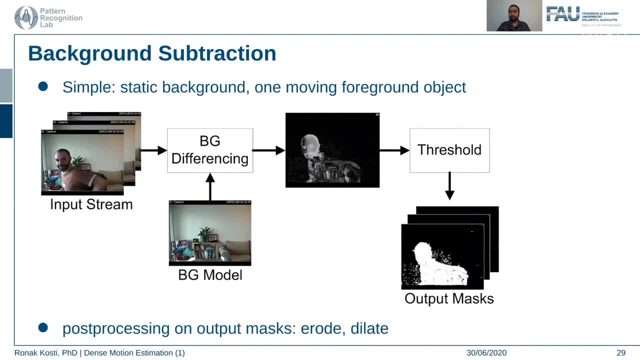 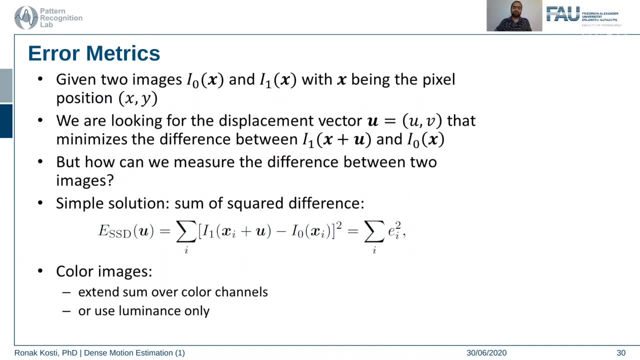 erosion, followed by dilation, which is basically closing, and you can remove this spurious noise from your generated masks. Okay, so how do we compute the errors? So what? Why do we need error maps, Error metrics? the main, the main, the main motivation to use error metrics is to find the differences. 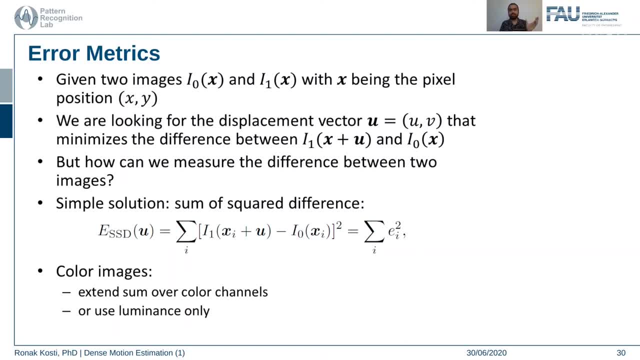 between to these successive frames or the video frames or these two successive images that you have for estimating motion. So let's say you have two different images: i0 and i1.. X shows the position of the pixel values there. Now we are, What we are interested in. 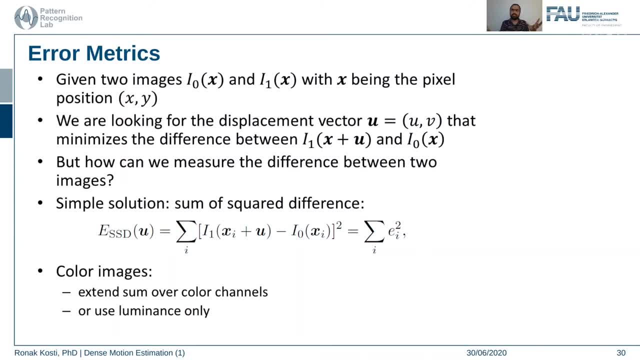 To find this translation of this one image towards the two to the other image, is finding a u vector which is u and v denotes, like the x and y directions, which minimizes the difference between the the i1 and i0. because if we are So, essentially what we are doing is we are converting this translational motion into. 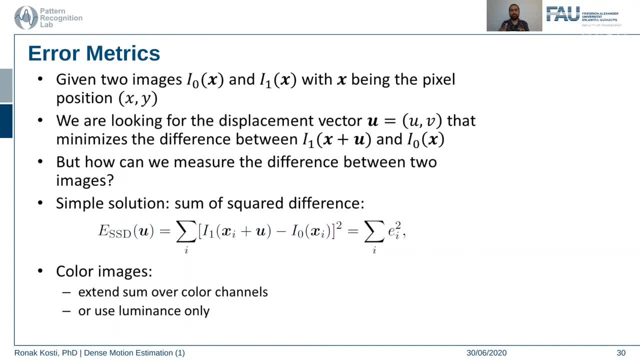 a minimization problem, Where We estimate the value of u such that it minimizes the differences between these two images, and that's our intention, right, in order to find this translation. But how can we measure these differences between two images? So that is where the error metrics come in. 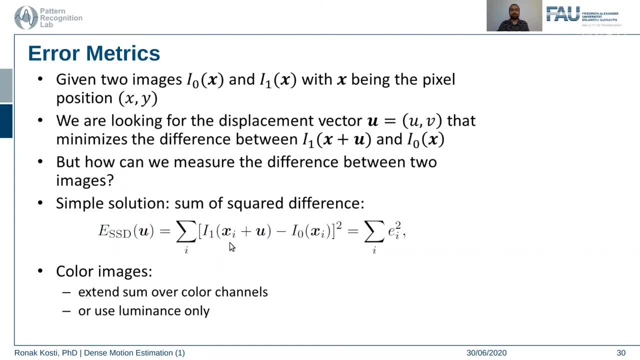 That's the motivation here. So you move your second image with a small motion, u, and you take a difference of those values with the original image And you accumulate in, you know, in a value which is called a sum of squared distances, And this will give you how much error, or the quantity in a quantitative sense, how much. 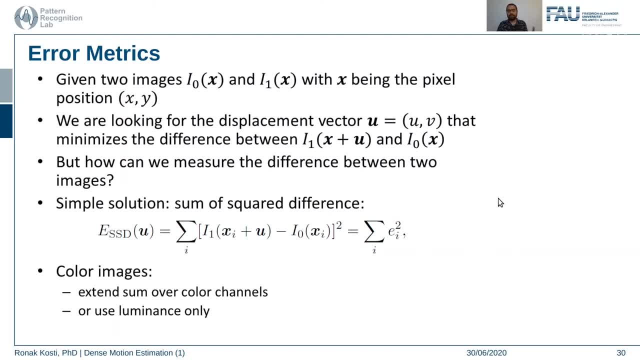 is the difference between these two images, And it gives you a reference value of how much you want to minimize this value. Ideally, you would prefer The best solution is: if the error is zero, then you have. It means that you have faithfully estimated the value of u. 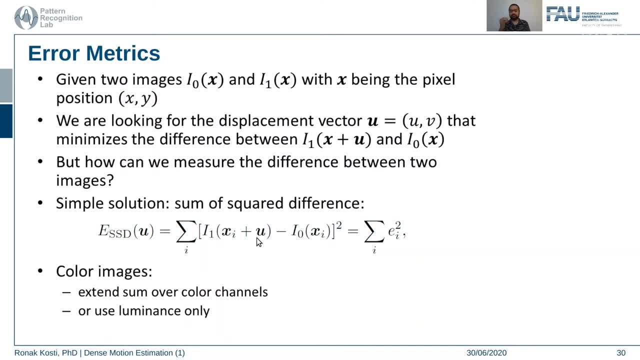 It's not a simple, straightforward Minimization problem, but the way we have formulated here is just finding in a finding the value of u through minimizing this error values Up until now. I Have to mention that we are assuming that all the images are black and white in our 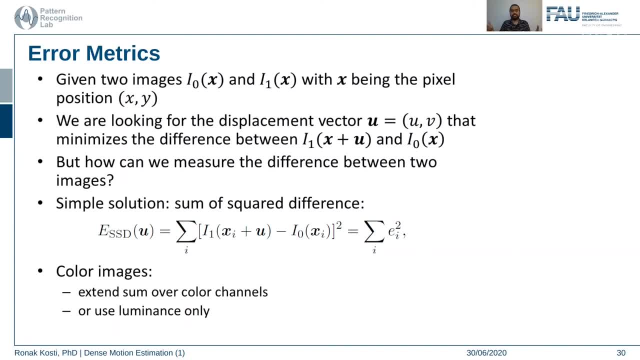 gray scale So that it's easier to compute these differences and the motions and optical flow. However, you can just use all the image channels and aggregate their sums or the errors, or even you can use or transform this color image into y, c, b, c, r or y u v image. 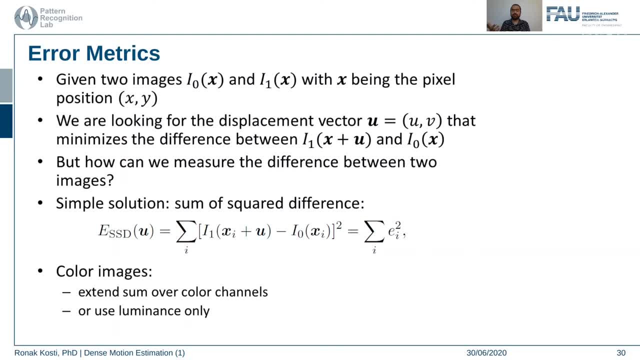 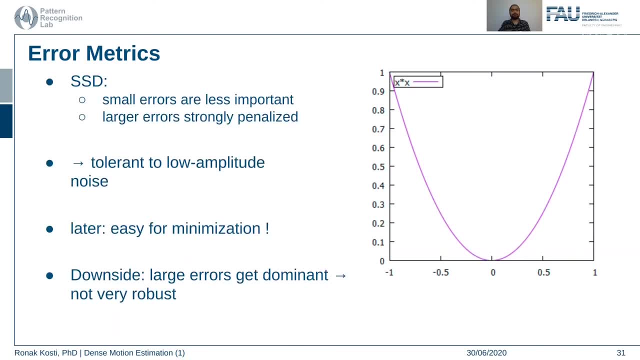 Image color space, And you can use the luminance or the intensity values to compute this differences, Which is also fine. Okay, so how do these s s d metric behave? So they have smaller errors for pixels which have moved in a smaller distance value, whereas 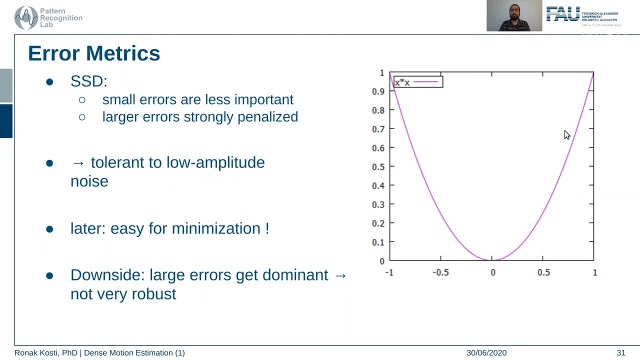 for pixels which are moving too far, too much, They have a larger errors and these larger errors, as you can see, are increasing exponentially. So basically, by looking at this curve, you can see that the sum of square distances is tolerant towards less important or lower value of the errors. 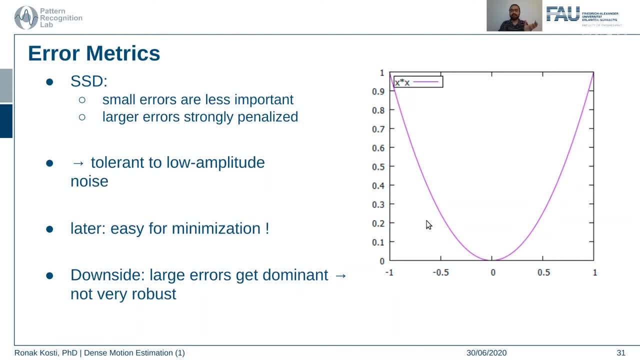 So if you have moved from five pixels to six pixels, it the error is not too high. But if If you have moved from 20 to 30 pixels, the error is much higher and the error metric is much higher. So this is easier for minimization. but the biggest down size is that the it's not very 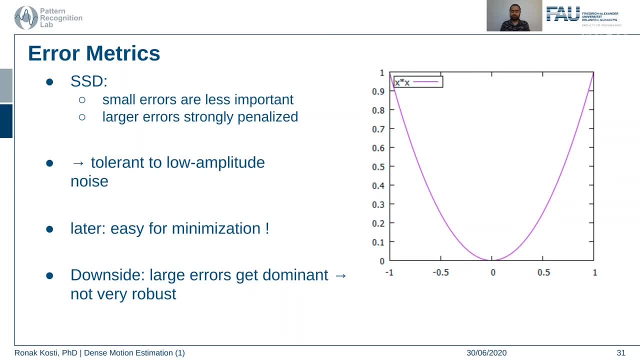 robust. For example, there are a lot of pixels which have moved or which gives very small error. Let's say that there are 50 pixels Which give which more or which give error, pixel value of one. So you have 50 as your value for the the error. 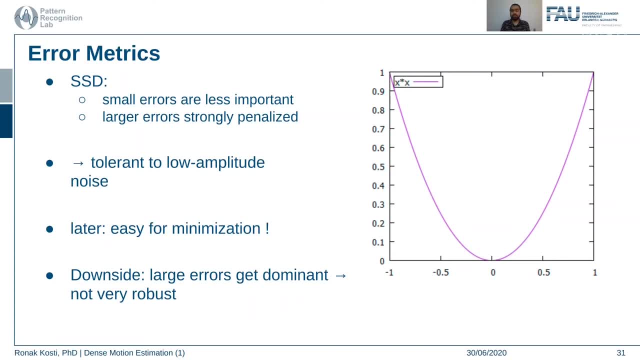 Right, Whereas there is a pixel which has moved in, moved by 60 pixels, and that one pixel itself will give you an error value of 60.. So a combination of 50 small error values is lower than just single large error, and therefore Larger errors dominate the SSD metric. 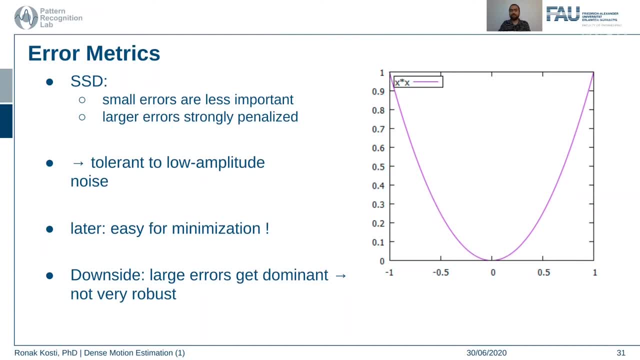 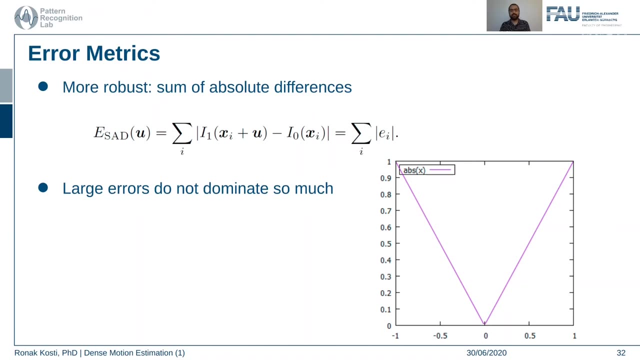 And therefore we can say that this metric is not robust for considering this- differences in the errors. So we need a bit more robust metric. Instead of doing a sum of squared distances, we can take the sum of absolute differences. This gives us a bit more robust. 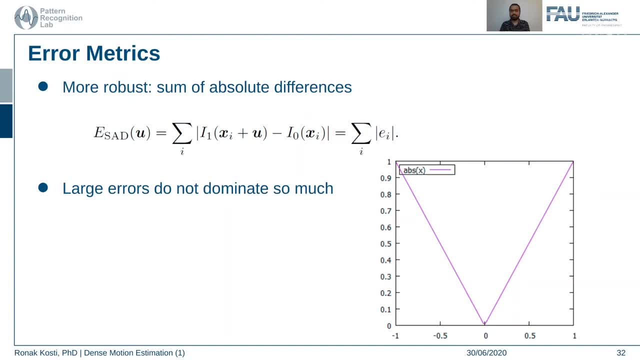 As compared. this gives us a bit more robustness as compared to the SSD metric. Why? Because you can see the shape of the curve here, that the error does not grow exponentially, It grows linearly. So large errors do not dominate as much as they did for the SSD metric. 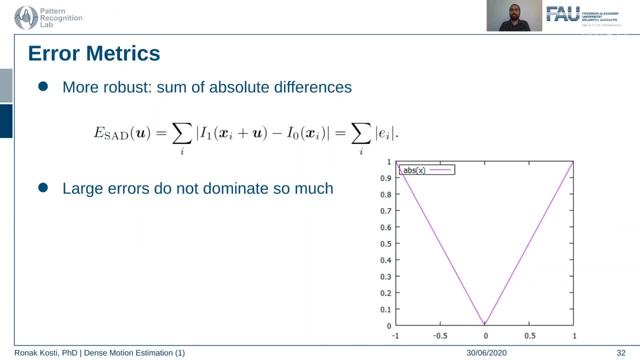 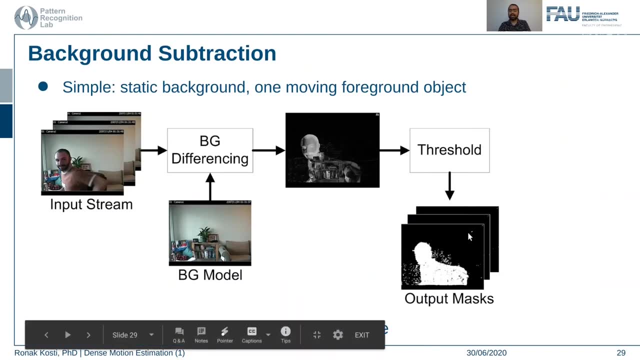 However, they still do dominate and there might be some noise. For example, Here we saw that there are some spurious, Spurious Noise in the background And these values can dominate or give large errors and we still do not want that they dominate in our error metric. 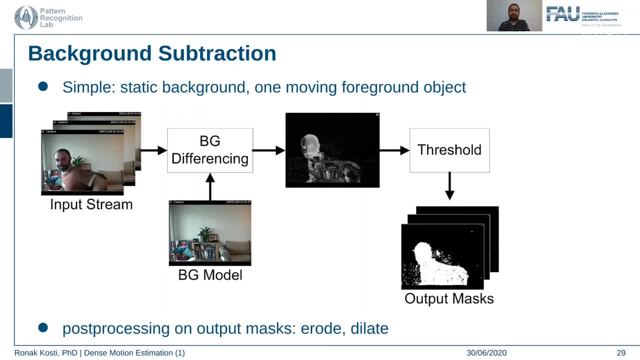 More specifically, what we want is that if there are error or the pixel values which are closer to our region of interest or farther from our region of interest, Both of these are error metrics for us. We don't want them to give two different values of error. 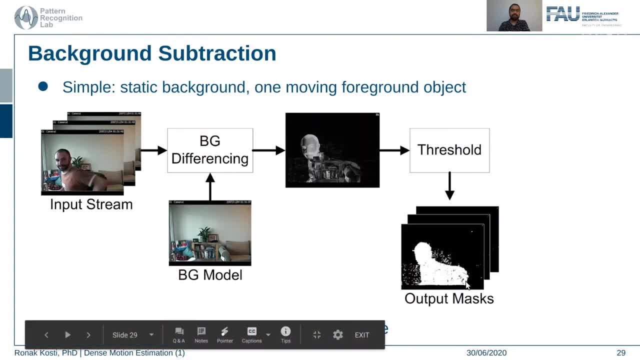 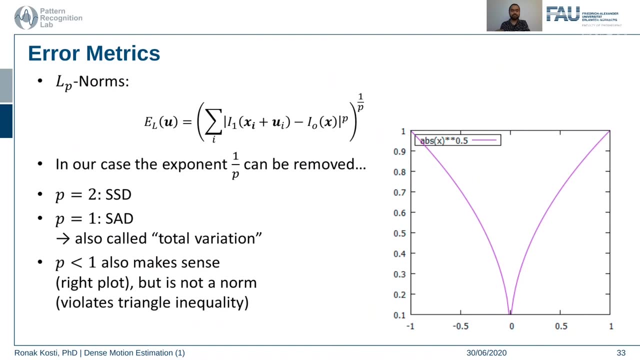 We want to set a threshold, that let's say we set a threshold that our region of interest is this mass and everything away from this mass. If there is an error, it gives us a constant error. So can we do that? That's the question. 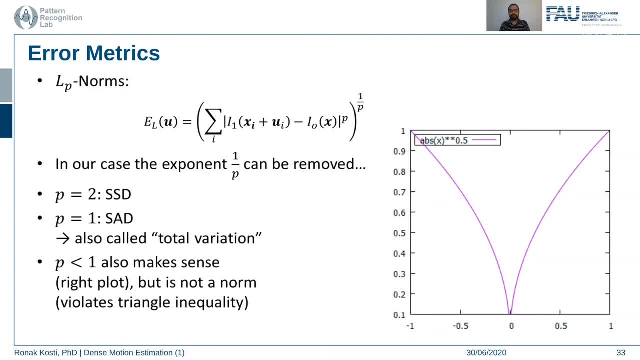 But before we talk about the solution- One of the potential solution until now- for SSD and SAD, these two norms are considered as LP norms. The generic form is written in this manner: If you take P equals to 2, it gets converted to SSD. 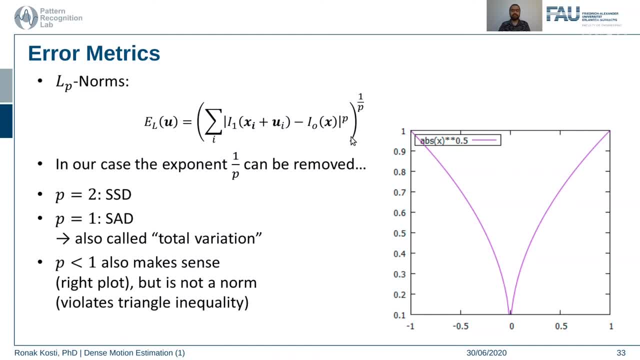 If you take P equals to 1, it gets converted into SAD. So we are seeing here that if you decrease the value or of P, you are making a curve which is Punishing larger errors very much slowly. So as you move more farther away, the larger errors are getting dominated more slowly in. 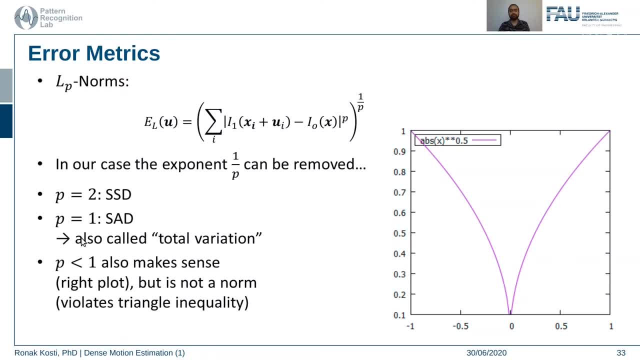 terms of when you decrease the value of P. This is called So it does. it makes sense and computationally or practically it is. it is what we want to achieve, Right, But it is not a norm. Those things will not be considered as norm. 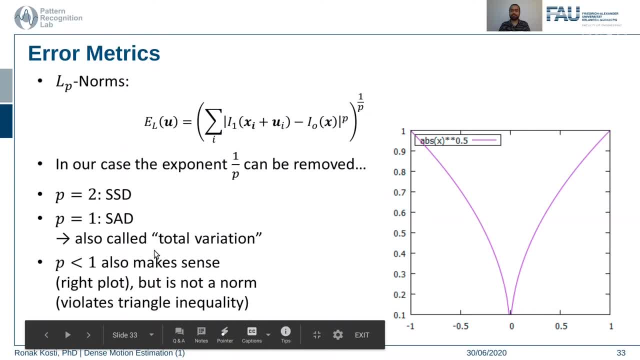 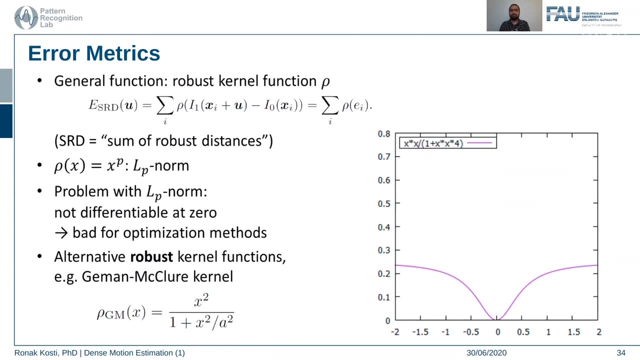 And this is some mathematical concept where, if P values are less than one, they are not considered norms. It's not directly relevant to our problem, but it is important to note. OK, So we were talking about some general, more robust functions which can help us give a 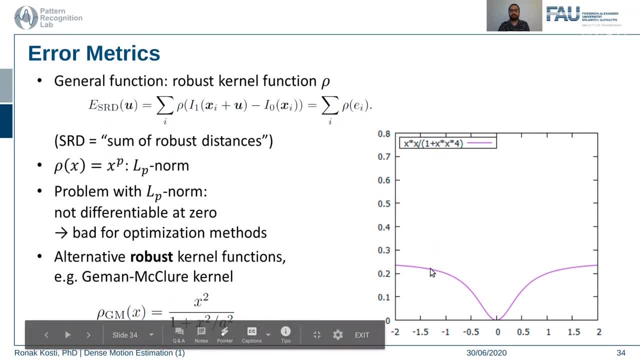 constant value of errors For P which are larger than a threshold value. Right, And this is in general called a general function, is called a sum of robust distances. What here we do is, After a certain distance, the errors, whether it is 50 pixels or 100 pixels. there the error. 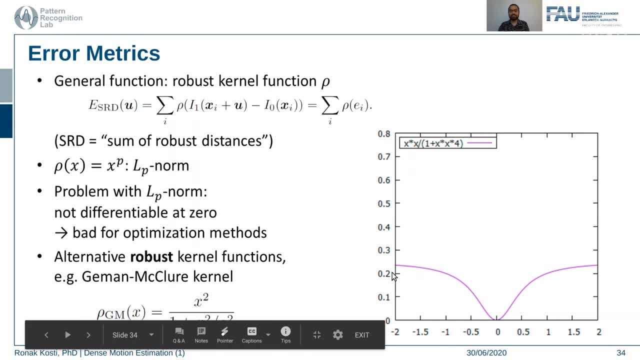 metric is penalized only with a fixed value. As you can see, the error is growing more slowly for larger distances And therefore we focus our interest in the lower error regions. And one of these robust kernel functions for generating the sum of robust distances is 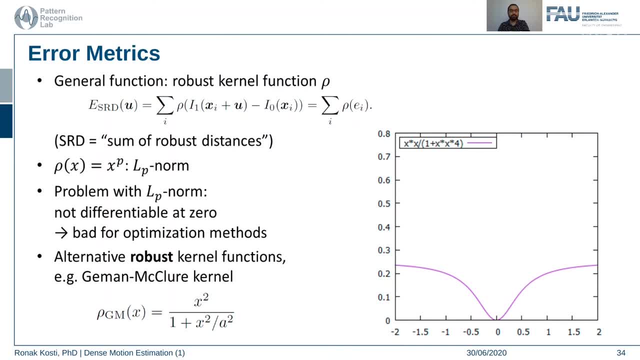 a Gaiman McClure kernel Here. if you plot this curve, it looks on something like on the right hand side. It's not exactly the same curve, but it looks. the shape is similar and this is what we want our error metric to behave like. 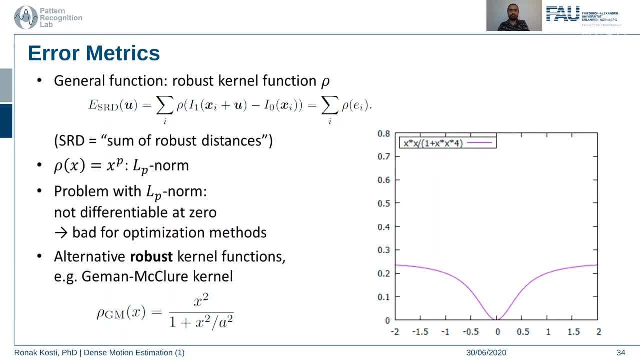 So, for example, if there is no, if the error value is zero, that is ideally what we want. But if the error values are higher for lower movement of the pixel, we don't want them to be punished or their values to be too high. And if the pixel movements are very high, we don't want those values to dominate our error. 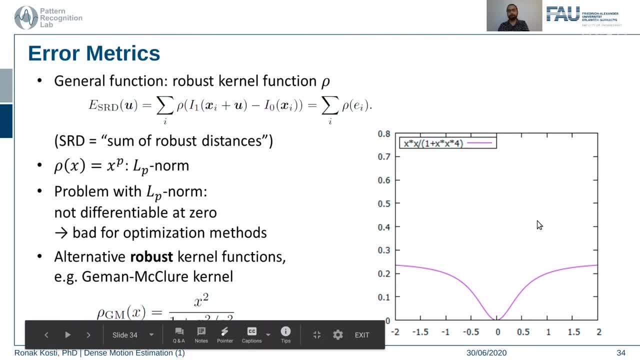 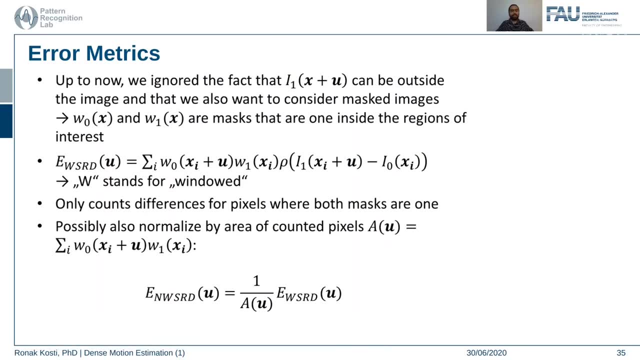 metric And this curve, This kind of curve, Takes care of it. OK, up until now we have not considered or not focused our attention to the region of interest that we are focused in, So it is quite possible that there are some regions of image in one frame which are not. 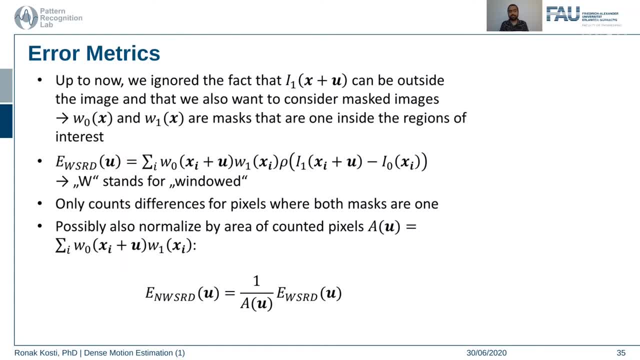 present in the other or they go outside of the image, basically, And in those cases, basically the errors will jump to a large value value. So instead of doing that, what we do is we generate masks. So W0 is a mask for I0 image and W1 is a mask for I1 image. Remember that these two images could be two frames. 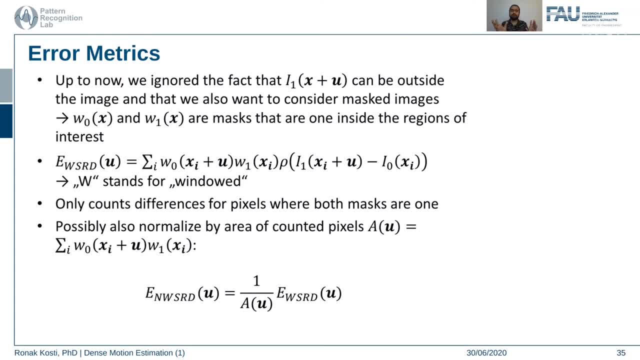 set in succession, or two animated, or two frames of animation video or something like that, And what we call here W is a windowed, squared, robust distance. What happens here is in each of these images. we apply this mask over the image so that our focus is only on the object. 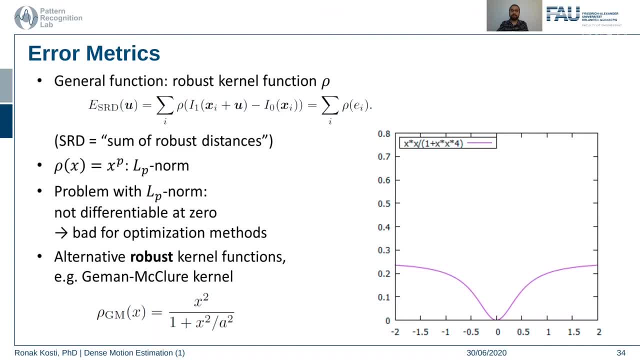 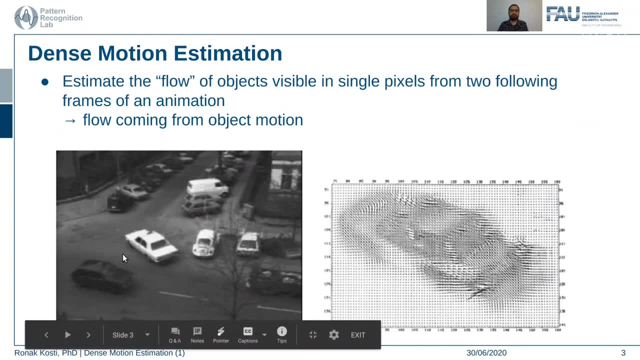 of interest. Let's say, for example, in our initial example, where we want to estimate this motion of this car, for example, then we create a windowed function here which only takes or considers value for this car and neglects every other pixel value. Essentially what we have to. 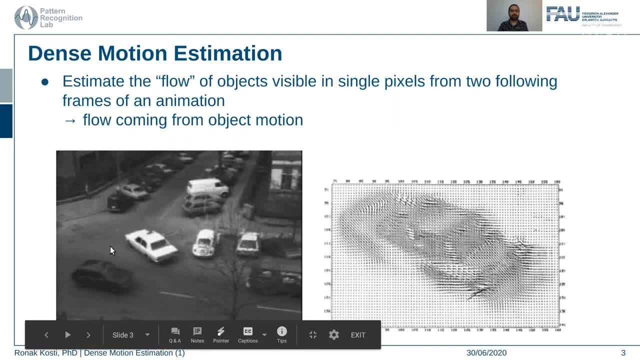 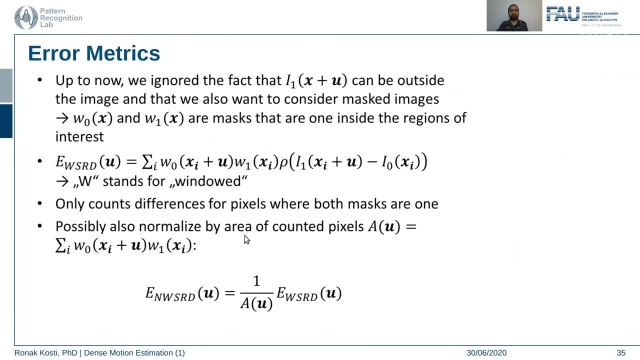 do is we have to multiply this whole image with a windowed function where every other pixel will be considered zero value, And that is what the W stands for: windowed, squared, robust distance. Here you can see that we apply the mask over the 0th image or in the. 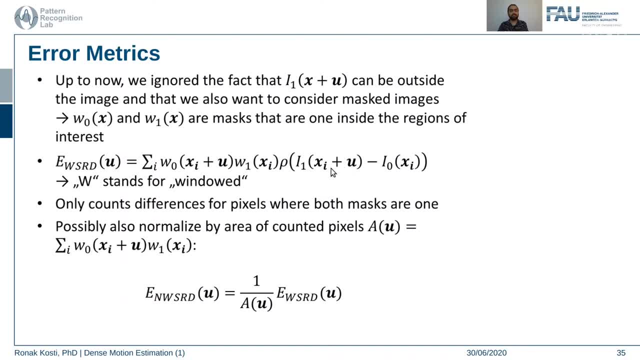 first image And then you compute the robust distances, essentially counting the differences only where these pixels are, only where these masks are present. So we are focusing our interest in those regions of the image where we want to track a person or an object and things like that. 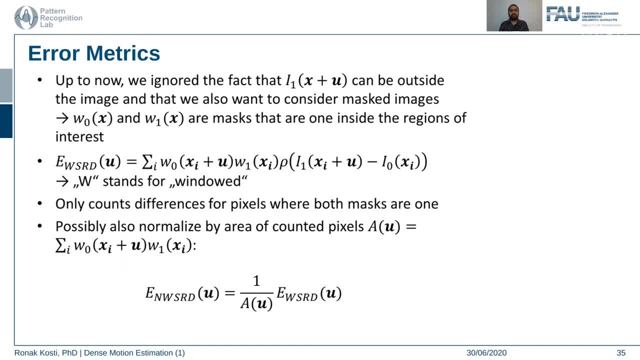 But it's possible in this case also that the number of pixels are higher and because of it, the error grows unboundedly and we can have a large error value In order to just keep it at the lowest. what we do is we divide our error with the area. 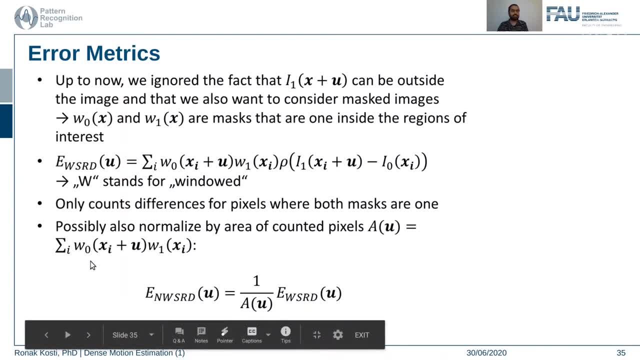 of the mask And that's how basically it's a, it's a multiplication of these two masks which shows that it will be so. a is an area of the overlap of these two months in these two images And therefore we are normalizing the value of this error metric so that it 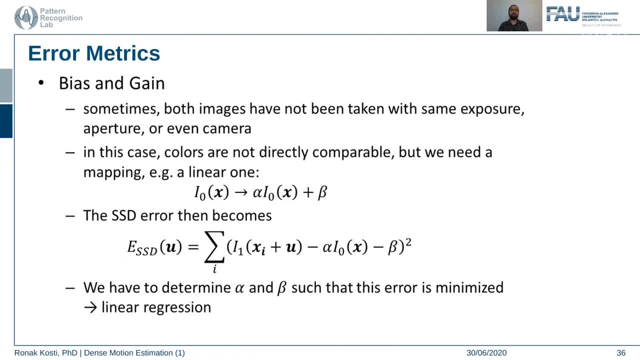 does not grow Unboundedly. Okay. so what's the advantage of using robust distances is, sometimes images are not taken with the same exposure. the sometimes the upper aperture changes, or even the camera changes, or the time of the day when you want to take the image changes, and so on and so 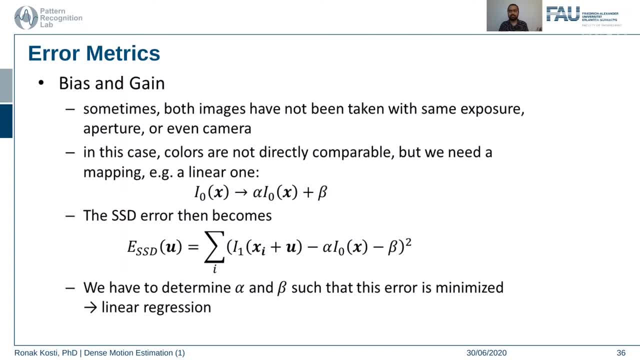 forth. So in this case, maybe it becomes more cloudy, maybe there is a sun coming out because of the clouds and things like that. So there are things which are not in our control. However, in these cases, it's not easy to compute or compare the images in their color spaces. 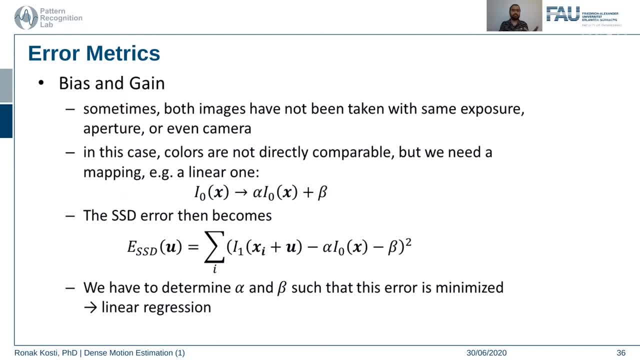 So we need a better mapping that can map over this changed luminance or a changed exposure or different camera image to the original one. right, we need a kind of a linear map And there If we assume that I not is transformed to alpha, i not plus beta, then the SSD error. 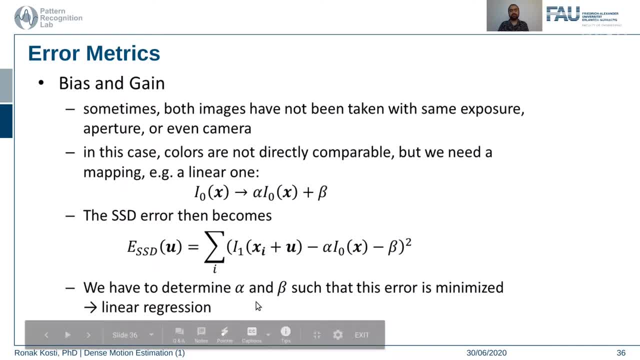 will become something like this. However, here we have to determine alpha and beta such that this error is minimized. Now it's like a minimization of the minimization problem. So we are a bit complicating our error estimation, or motion, motion, motion estimation, by complicating. 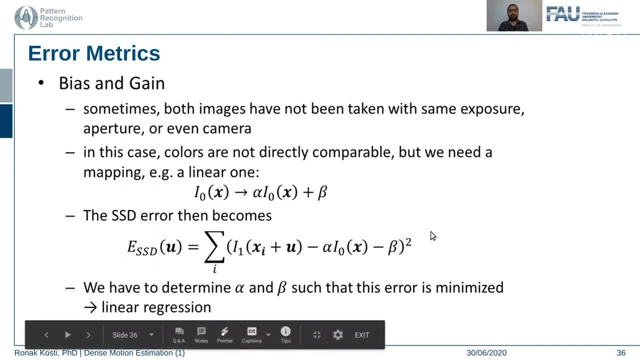 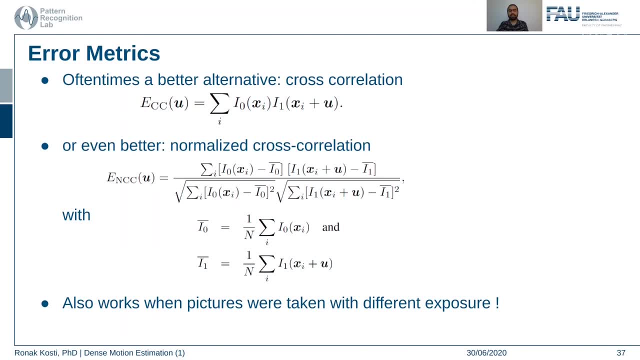 our error metric here. First we have to estimate alpha and beta and then we have to estimate you. So it's like a minimization of a minimization problem which makes it a bit more complicated. So a simpler, more direct solution is to directly use a cross correlation between the two images. 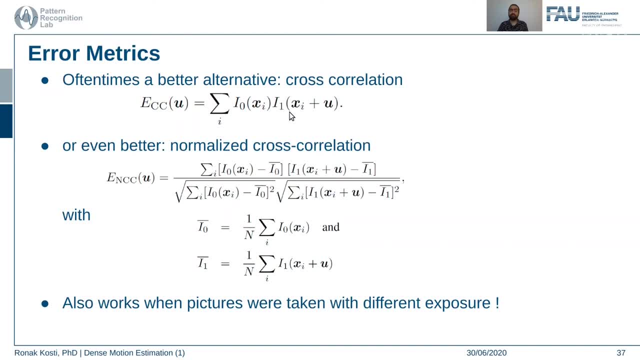 So we have seen what a cross correlation means. We have also seen what autocorrelation means: Cross correlation. why the reason the term cross correlation here is used is because it is not with the same image. It's an image, It's a correlation between two images. 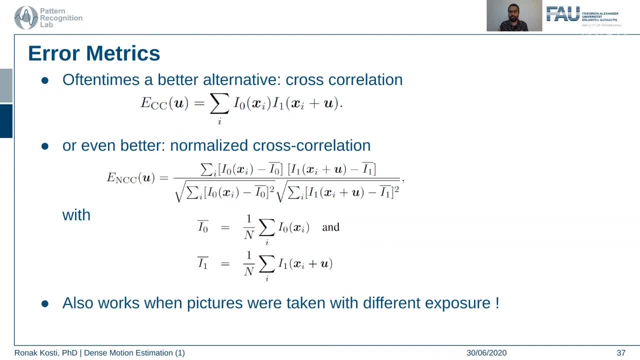 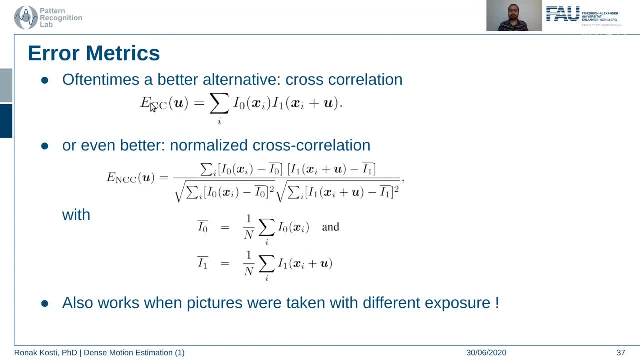 and essentially, instead of minimizing this cross correlation, what we want to do is have a maximum value of this cross correlation. Why? Because if the cross correlation value is maximum, It means that images are overlapping quite perfectly, or the way you want them to be. 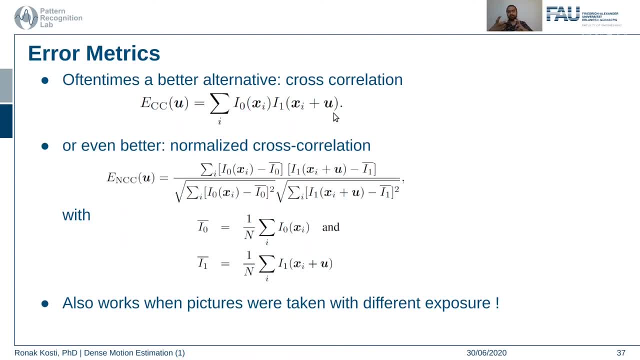 to find this correlation or to find this mapping between, or to join or things like that for the motion. So in that case your U value is estimated. So basically, that's what a cross correlation does. Even with cross correlation, you can have a normalization issues.